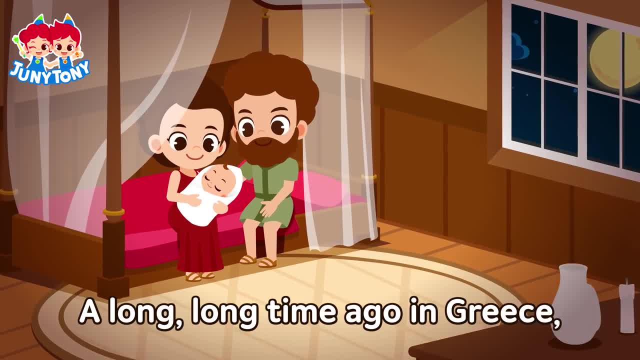 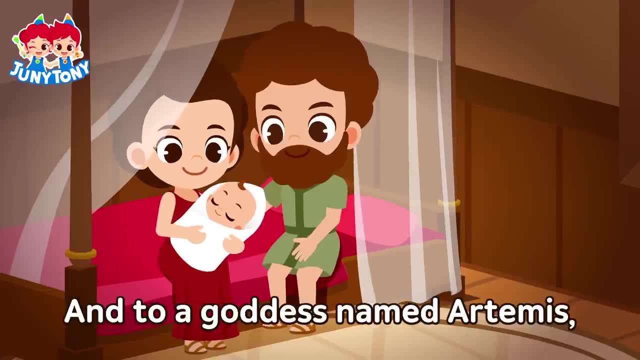 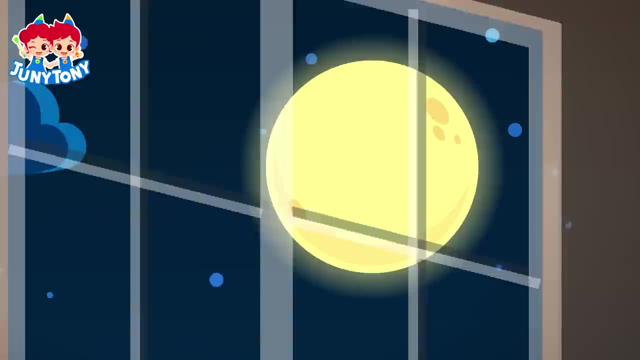 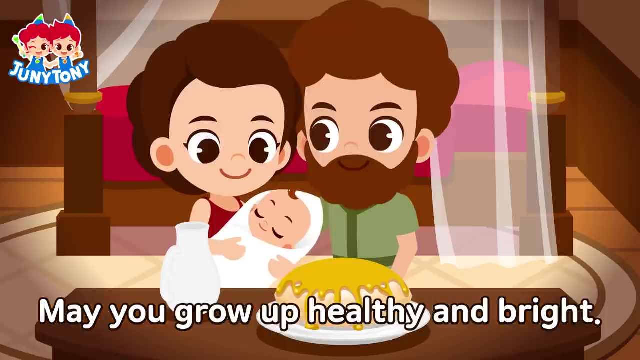 Junie, Tony will let you go. A long, long time ago in Greece, They baked a cake for a newborn baby And to a goddess named Artemis. They baked a cake to make a wish. May you grow up healthy and bright. May you be shining like moonlight. 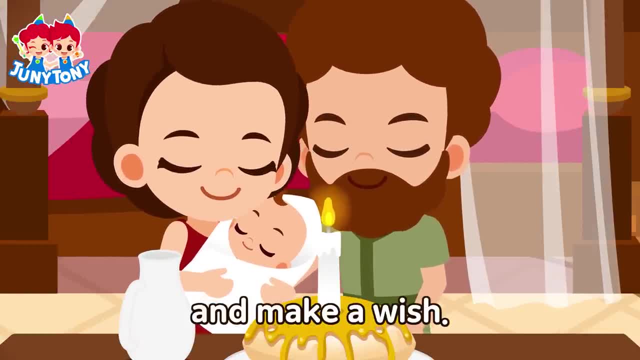 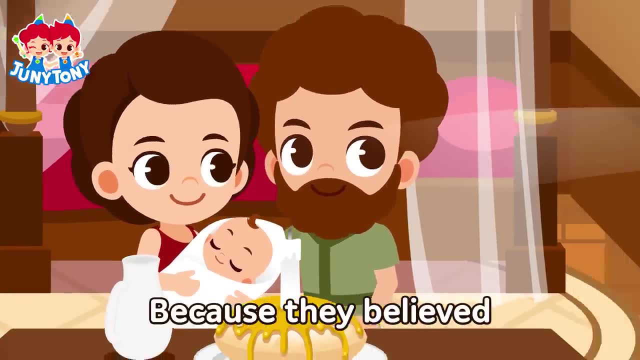 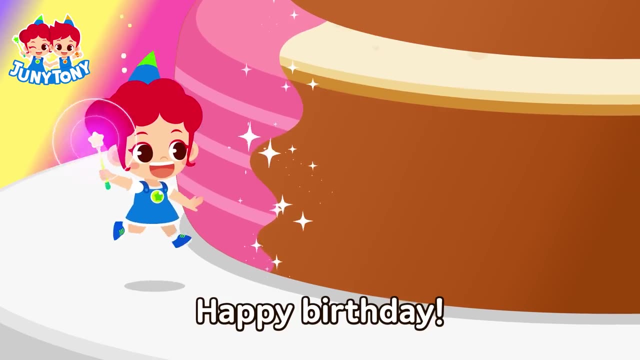 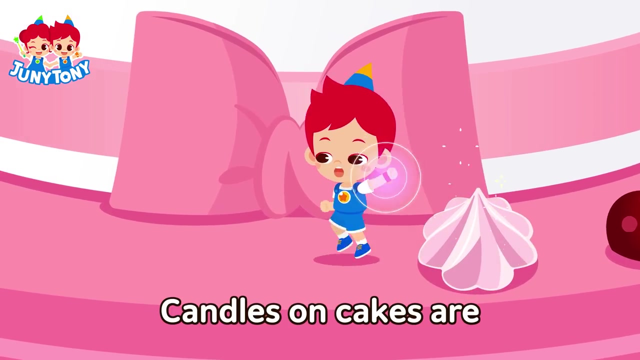 May you be shining like moonlight. May you be shining like moonlight. Put candles on a cake and make a wish. I wish you the best And blow out the candles, Because they believed that their wishes will come true. Happy birthday. Happy birthday, Candles on cakes are because of love. 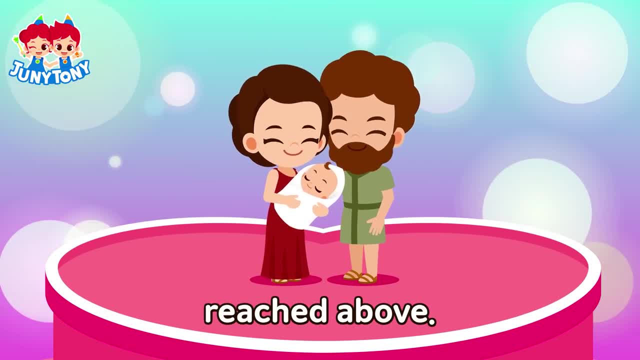 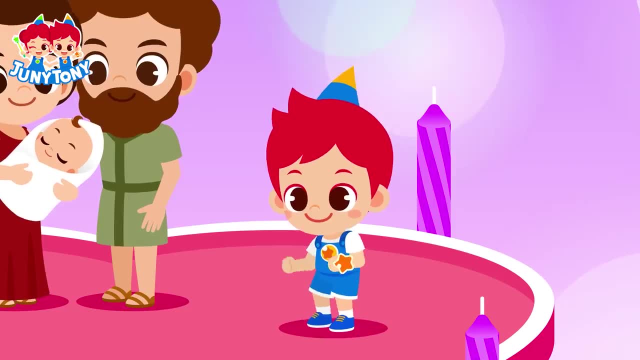 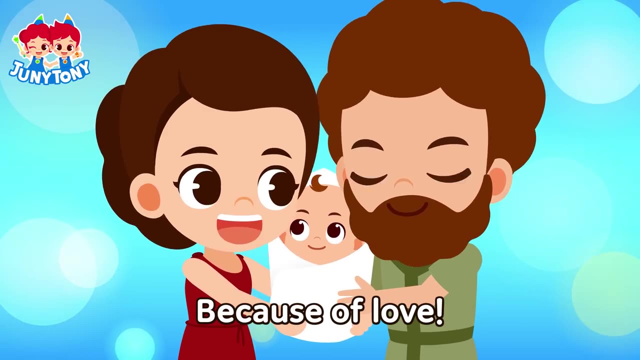 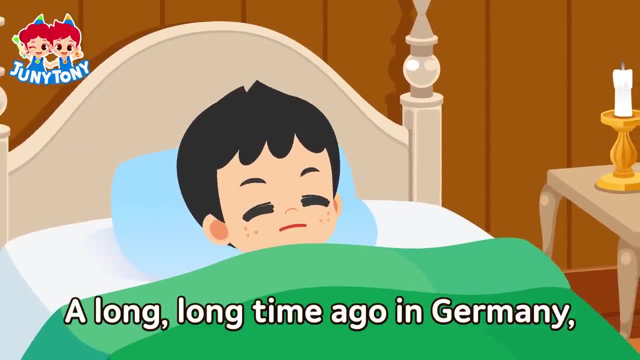 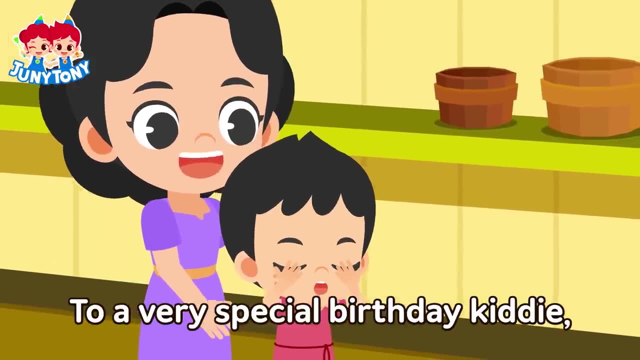 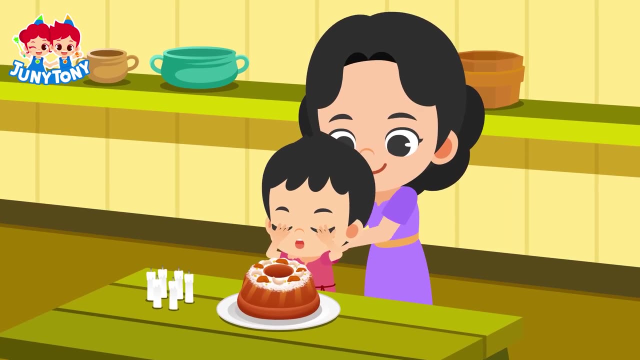 Because of love. A long, long time ago in Germany They gave a cake on the birthday morning To a baby girl, To a baby girl, And a very special birthday kitty. A homemade cake was a birthday present, A very special birthday kitty. 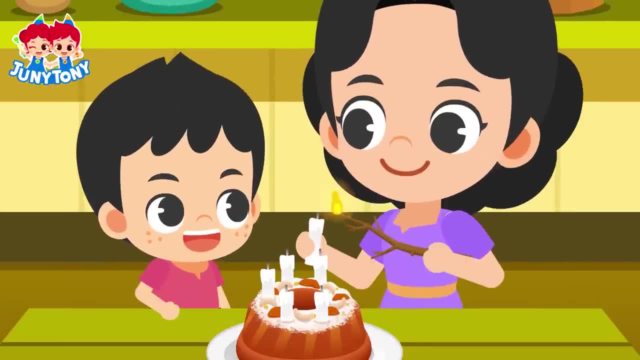 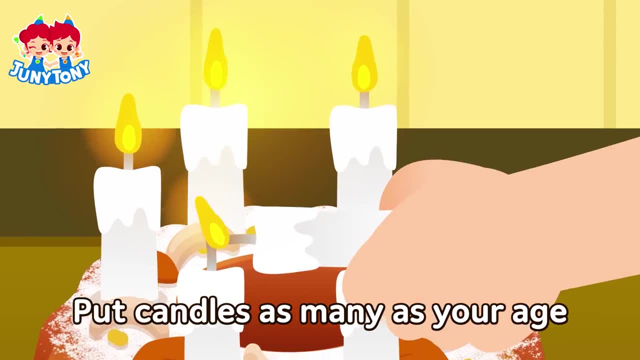 A homemade cake was a birthday present. May you have a wise insight. May you be shining like starlight. May you be shining like starlight. Put candles as many as your age, And another candle on the cake, And another candle on the cake. It's a Light of Light. 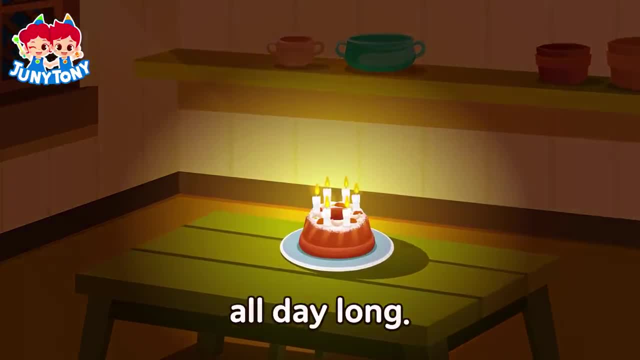 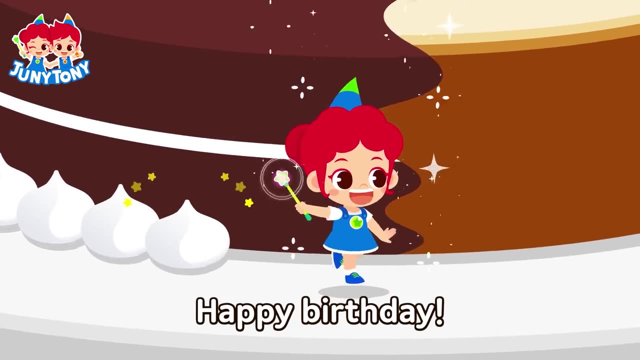 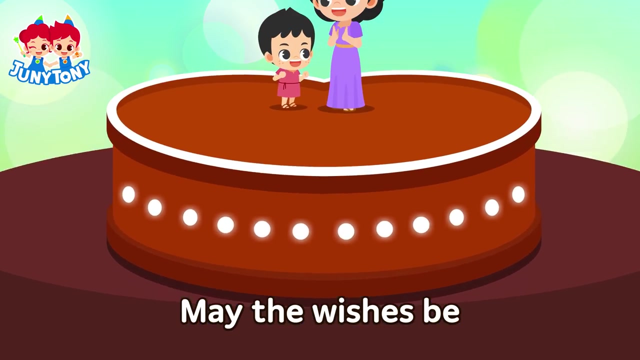 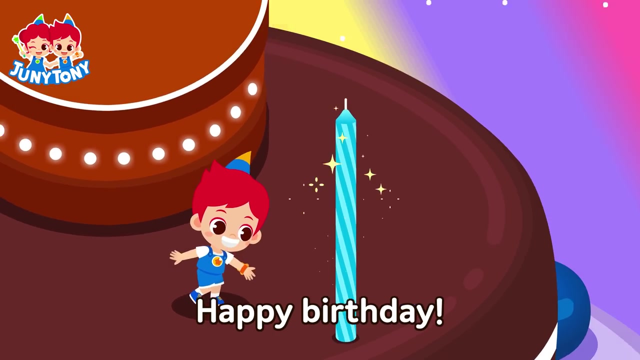 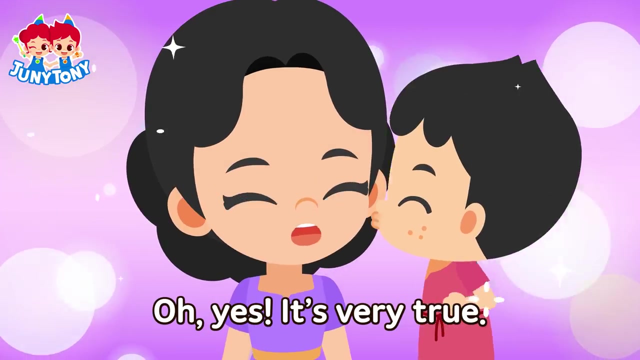 And they lit, And they lit all the candles, The candles all day long. Happy birthday, Happy birthday. Candles on cakes are because of love. They deliciously reach the above. Happy birthday, Happy birthday Candles on cakes are because of you. Oh yes, it's very true.